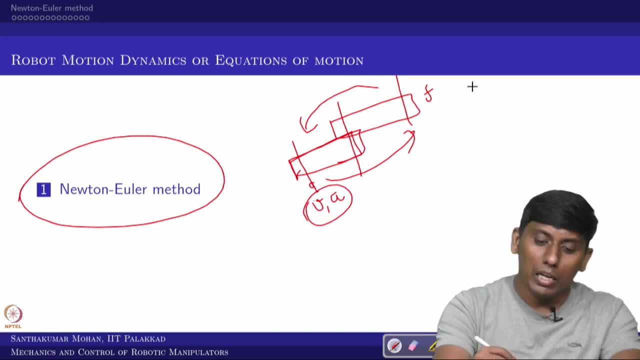 can see that the mass is actually like part of the body, Part of link. So the link I is having actually, like you can say, I axis and I plus 1 axis, right? So in the sense we are not talking about the inertia on a joint. So please be clear the 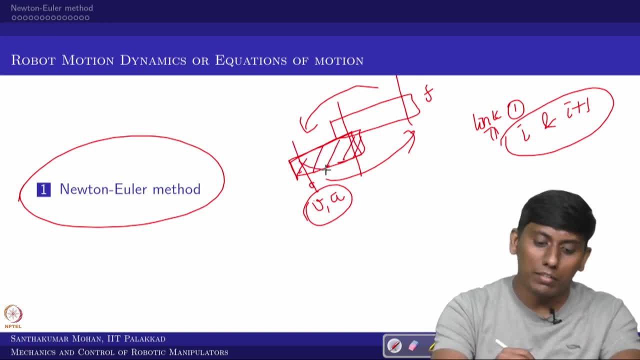 initial forces are due to the link or the mass which is pertaining, So that we would be clarifying, and then we will actually like go the velocity propagation and acceleration propagation from one to the other. So in the sense we would be doing 3 stage process, So that 3 stage process is actually. 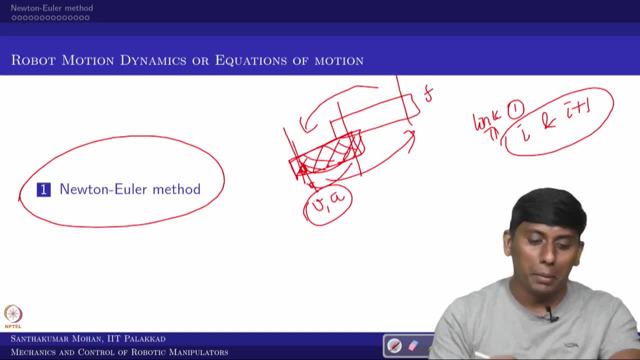 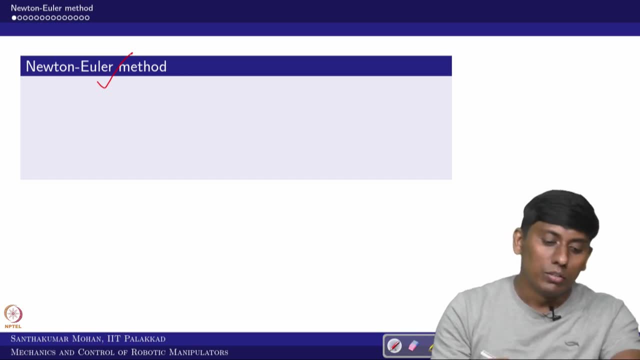 like what Newton Euler method called iterative one, or you can say iterative Newton Euler method. So now we will go, the generalized Newton Euler. So where this is actually like, based on the linear momentum and angular momentum. The angular momentum would brought from the Euler equation and the linear momentum brought by the Newton's equation. So now the Newton's. 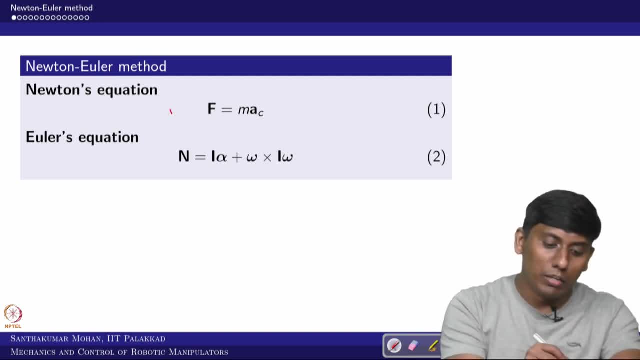 equation and the you can say Euler equation, the simplified Euler equation we are going to use. So where Mac- so here you can see this- Ac is the linear acceleration of the mass at centroid, So where I is actually like initial tensor and omega is actually like angular velocity. 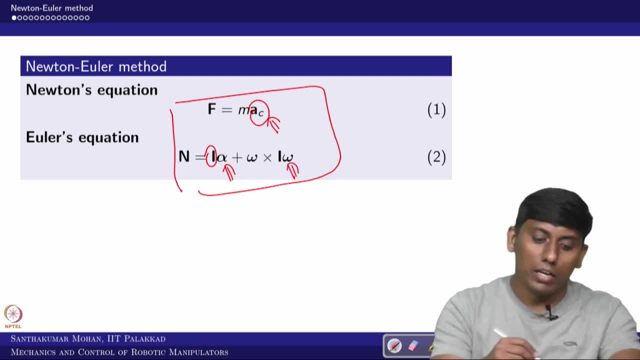 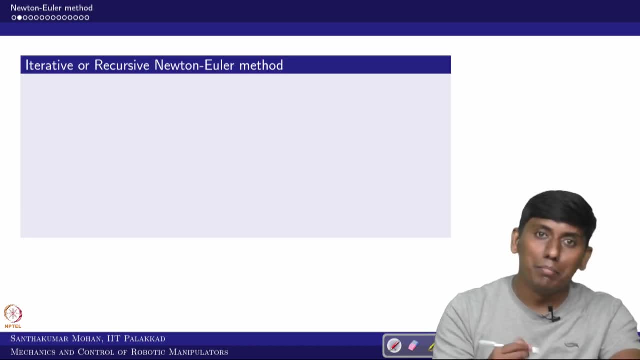 and alpha is, you can say, angular acceleration, and mass is actually like the link mass. So now, based on this equation, what one can actually like? try to see, We can make a iterative one. so here iterative is actually like different, so what that means. so we will actually like. 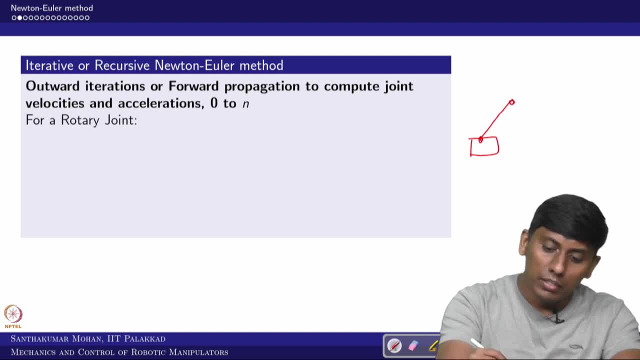 start. this is the base. So I am actually like trying to show That these are number of bodies, So we can actually see that the base velocities- so angular velocity, you can say acceleration, or alpha also 0, all are zeros. So this is all zero. 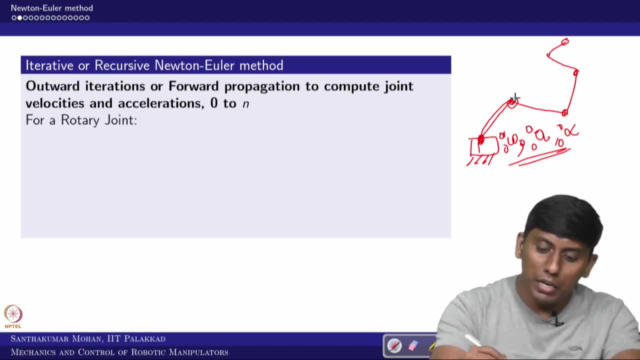 or else so in the sense. So every time there is a t, there is always a t. okay, so that's here. I can actually like go first frame, second frame, third frame and fourth frame, fifth frame, to end frame, right. 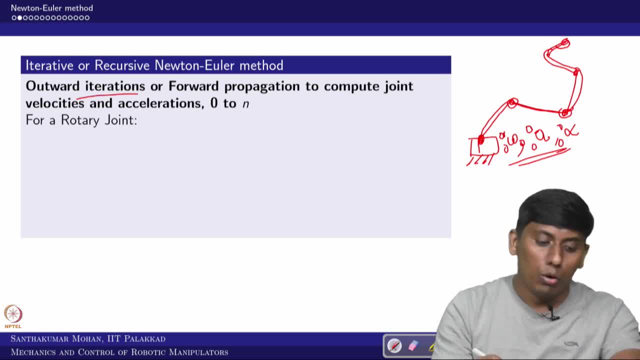 In the sense what I can do. I can actually like do outward iteration or forward propagation to compute joint velocities. okay, So corresponding joint velocities I can calculate with the help of whatever the equation which we derived In the sense omega i plus 1 to i plus 1. we know like already it is r i plus 1 to i, omega. 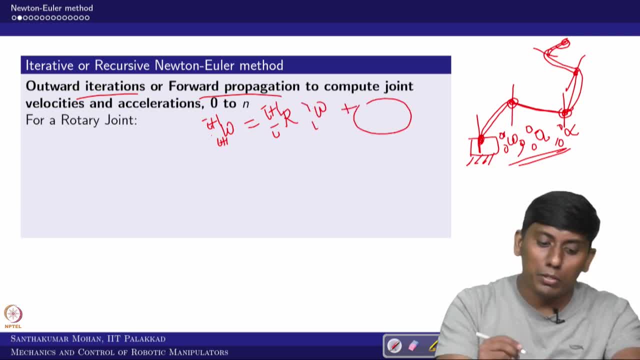 i, i. if it is a rotary joint, it would be added. if it is a prismatic joint, not, So similarly, alpha also. you can actually like get it So here. what addition will be there? This is actually like angular velocity, the similar way angular acceleration component. 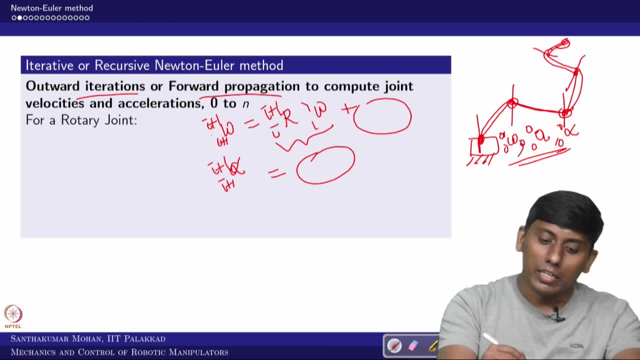 of previous joint would be there. further, the current angular velocity or in the sense, current active joint angular velocity, which would be interact with the previous joint angular velocity, because it is a same part of link. So that would give a gyroscopic effect. So that would be added okay. 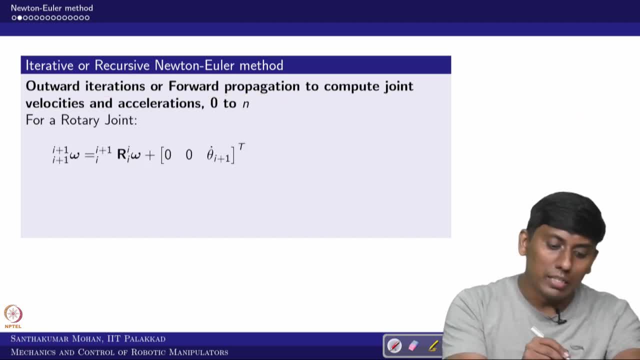 So, in the sense, what we are trying to do, we are trying to compute the- you can say angular velocity and as well as angular acceleration. So you can see the angular acceleration, previous joint angular acceleration. further you can see the gyroscopic effect In addition to that, the active- you can say joint acceleration. 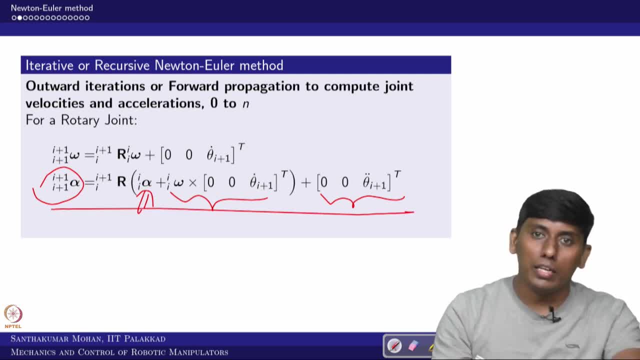 So these three are actually like coming into a picture. If it is actually like linear, the linear acceleration which we are interested is actually like this. So which would be? you can see one with come from the you can say slip acceleration of previous, then you can say tangential, then the radial, which we call centripetal, 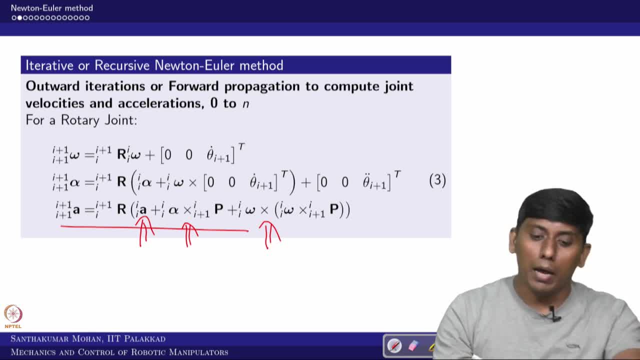 Some people even uses the Coriolis. The Coriolis will happen only if you have a interaction. this So in the sense you have a angular velocity and the linear velocity active in the sense this is having and there is a active linear joint. 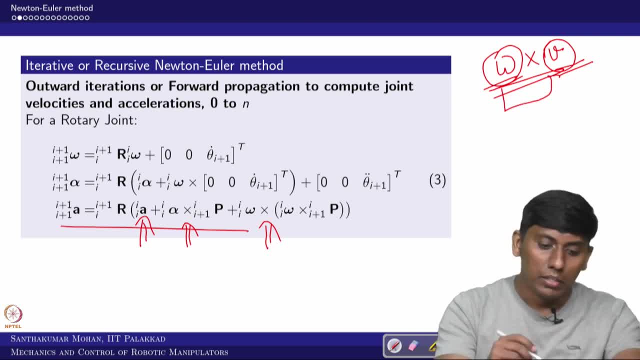 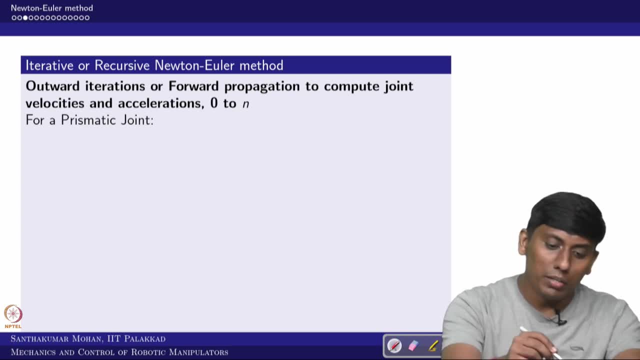 Then this Coriolis will come. otherwise there is no Coriolis component. So that is what we are actually like: trying to show The same thing. I am actually like writing in the prismatic joint. you can see prismatic joint. the angular velocity is very simple. 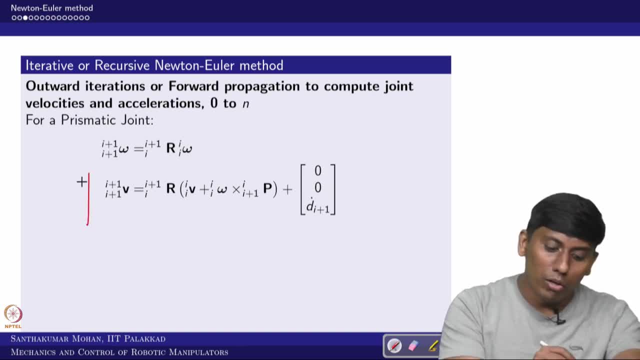 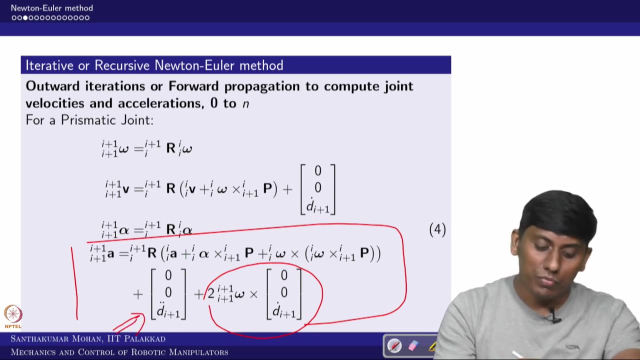 Similarly, angular acceleration also, like would be simple, But the velocity component you can recall because this would be useful further on. okay, So this is the angular acceleration part and this is the linear acceleration part. The linear acceleration part: you can see the slip acceleration added, which is slip on the. 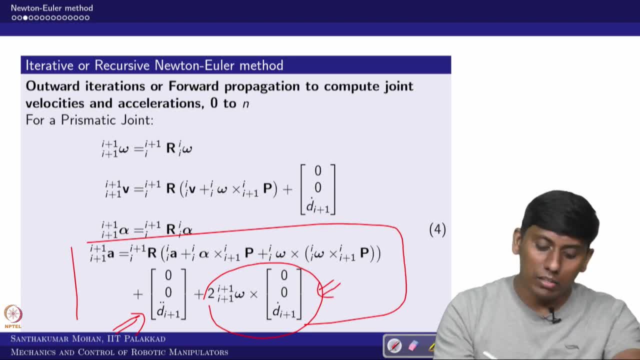 joint And you can see the Coriolis acceleration. The Coriolis acceleration is omega of i plus 1 to i plus 1 and d dot i plus 1.. So you can see the Coriolis acceleration. Okay, but this is D double dot, right? So you please make it this in your mind. So if it is a 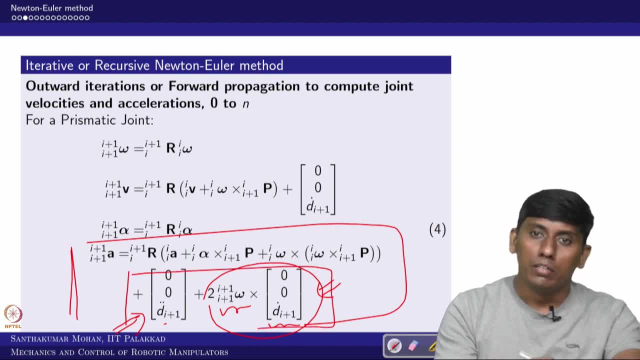 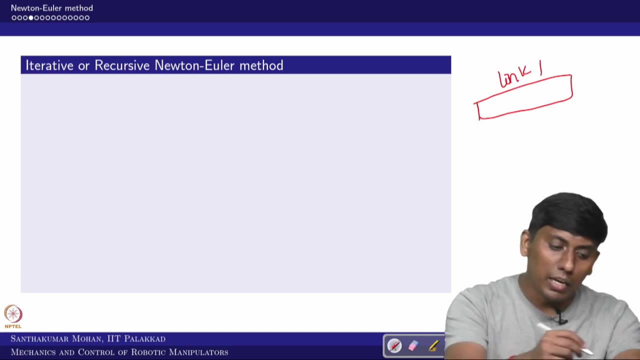 linear joint there would be two additional component will come further to what you can say, the previous joint accelerations all playing a picture. So now, in that sense, what one can do, for example, now I take link I, So link I would be having, you can say ith axis and I plus 1 axis, So I can calculate the angular acceleration. 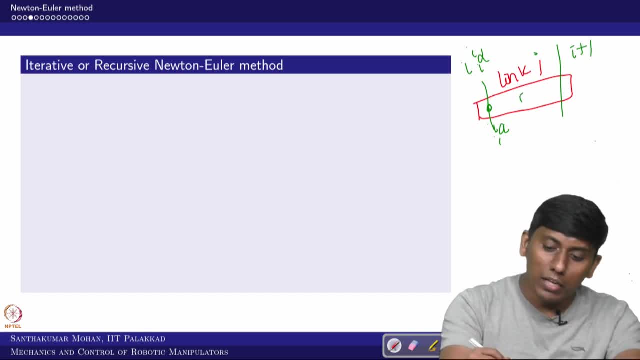 and linear acceleration: ok, but the mass would be concentrated somewhere, right? So I assume that this is actually like mass concentrated as a CG. So here only the inertia force would act, right. So, if you see, the acceleration is actually like happening here, like this: 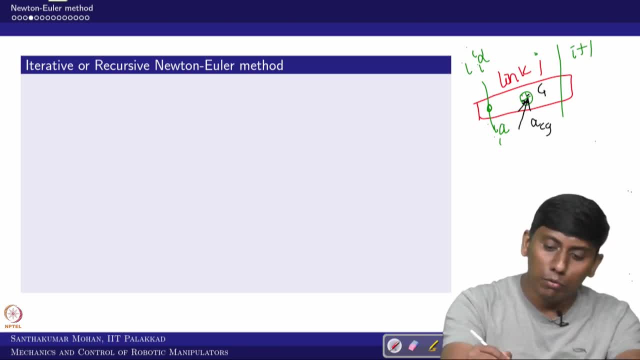 ok, So here only the force acting. here the force would be acting so just opposite to this, right. So M A CG would be acting So similarly alpha, so that you can say that torque would be actually like in this way, right, So this is what inertial torque. So these two we 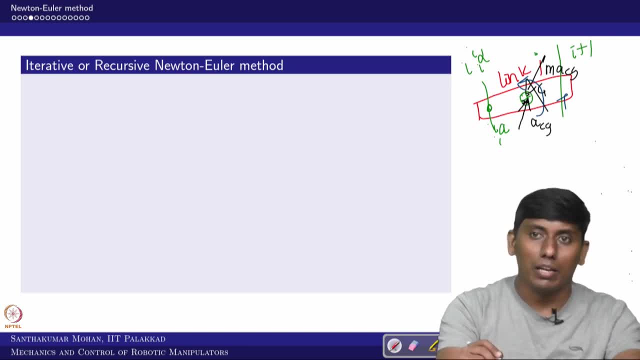 need to calculate. So now, what we are doing, we are not doing with joint, we are doing here link. So in the sense, what you need to know, you need to know the link: inertial force and moments. For that you need to know the link, centroidal acceleration. so for that what one can do, you, 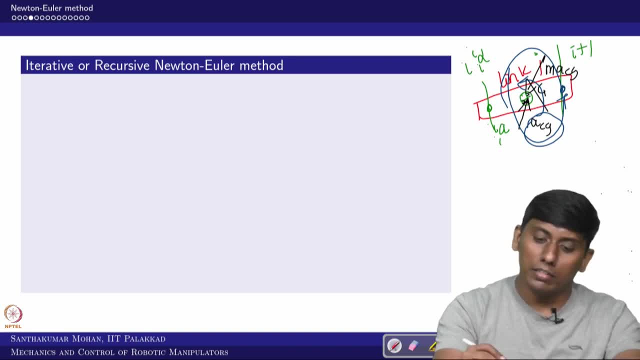 can actually like go from any one of the joint. the friffer is actually like forward propagation. so once you know A i to i, alpha i to i, so you can actually like go to A ci to i. okay, so that is what we are trying to do. so you can see inertial force and moment computation. 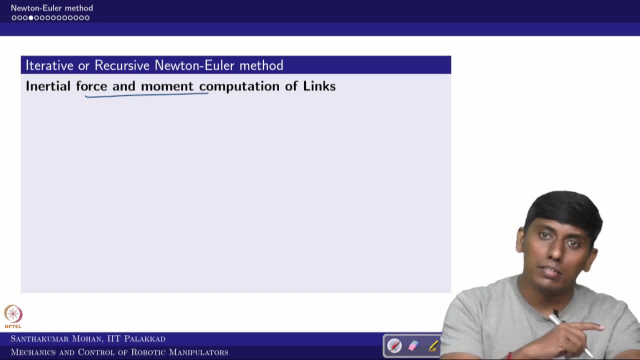 of link. so for what we have calculated of joints, please be clear. so this is of link. so if you have four joints, so how many links would be there? only three links would be there, right, because including ground four, so in the middle there would be three links. so for 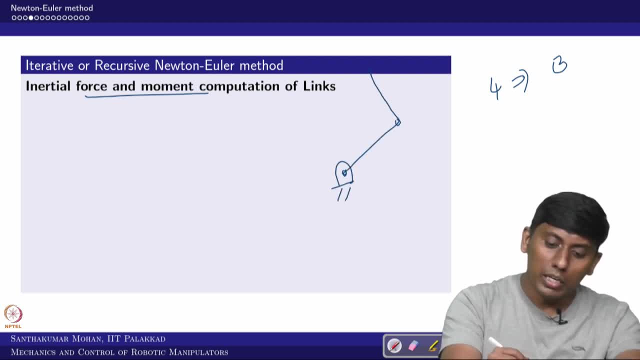 example you take a two hour serial manipulator, okay, so how many? you can say link, so the ground, so two. but in the sense there are two moving links, in the sense the centroid would be playing these two links. Okay, In the sense the link, inertial force and moments would be two components. so F you can say in: 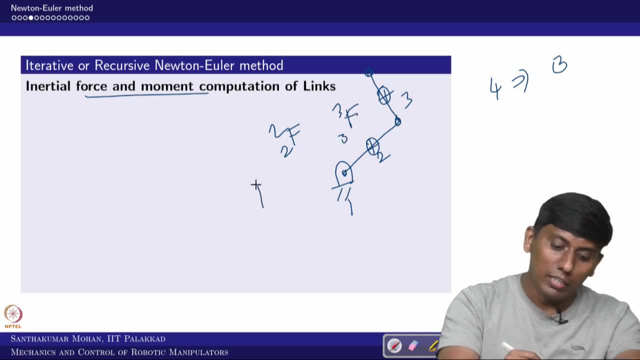 this case F 2, 2 and F 3, 3 and N 2, 2, N 3, 3. that is all will come. but how you are actually like denoting that is different. so we denote this one. so this is one C. so in the sense, 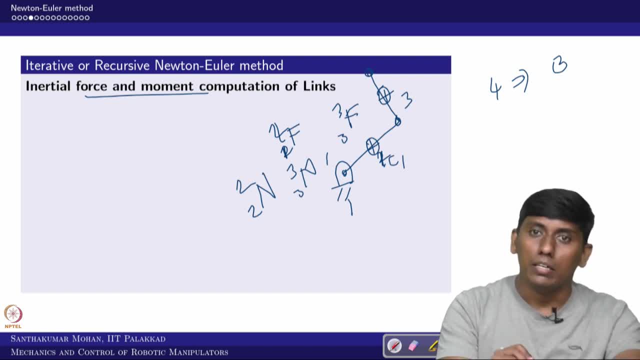 this is actually like one, that way you can actually like make it. This denotation is actually like we will come, the representation or how you are actually like approaching, but otherwise one supposed to know. we are calculating inertia forces and moments of a link where the acceleration we have calculated till the previous slide. 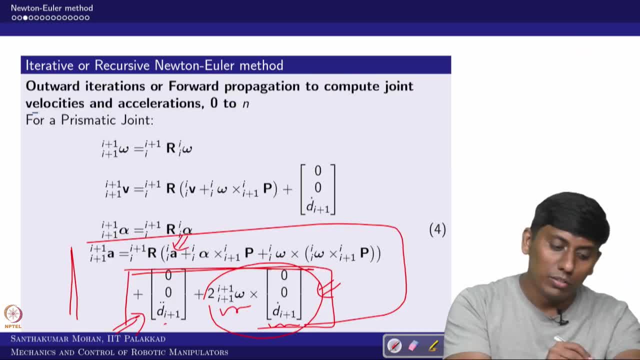 of you can say joints, right, so this is joint velocity and acceleration, Because several of time the students always confuse. so why you are calculating additionally one more velocity or one more acceleration? this is just to because you are having link which is consist of two joints. okay, that is what the idea we will see in example which. 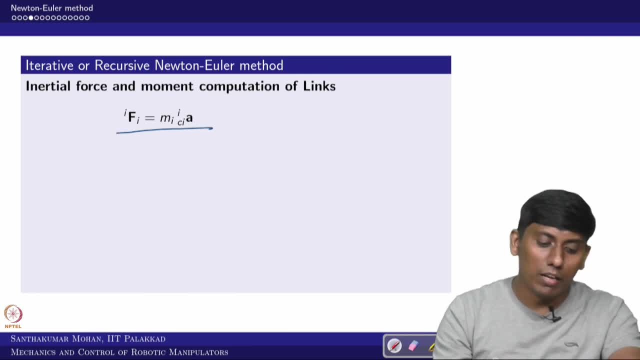 is very much clear to you. so now you can see the inertial force which we need to have, the- you can say, centroidal acceleration, linear acceleration, you should know. similarly, you can actually like calculate what we did the previous, because now it is actually like again. already you calculated your acceleration here, so you are actually like going here. so then, 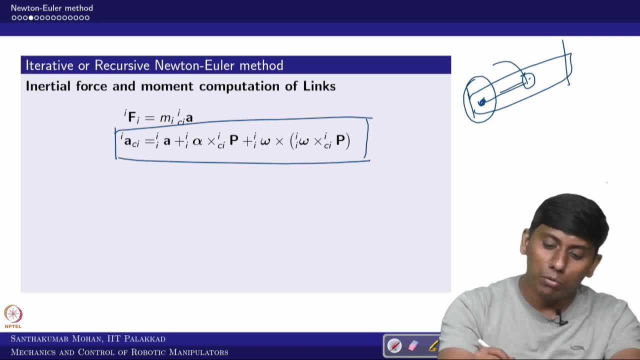 you can See, there would be a tangential acceleration, there would be a radial and there would be a same acceleration would go across, since these two are in the same frame. so you no need to actually like do any transformation. that is why you can see there is no, you can. 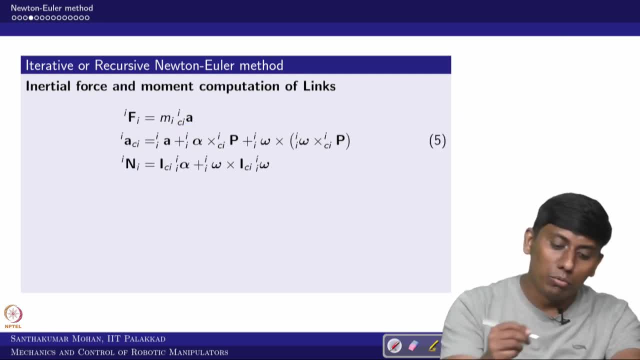 say rotation matrix on here, right? So the next one is actually: like you need to calculate the what you call angular moment at the inertial location so you can actually like see the inertia tensor at centroid. You calculate, then you can see that angular velocity and angular acceleration you will. 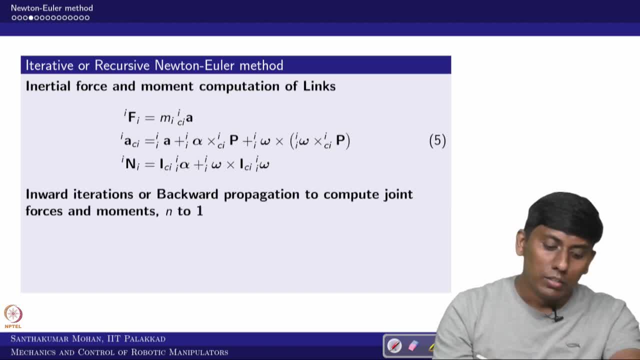 calculate these two, forces and moments. okay, so once you do this, so what we can actually like, do you can come back from n, because the end effect are the forces and the end effect are. you can say: I put e, the end effect are moments, are actually like, known to us. 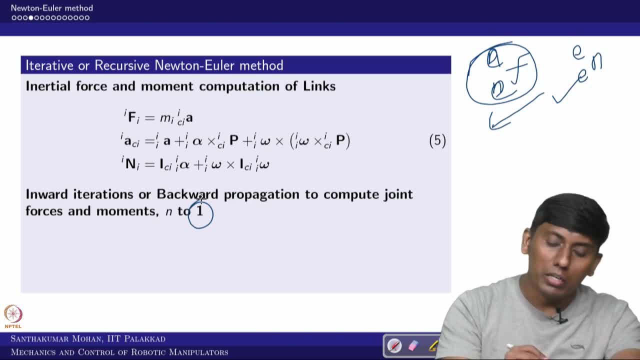 So then we can actually like come backward up to one, because one is the active joint. up to one, only active joints would be there. if you come to zero, that would be the base you can say support force and moment in addition to that, what this base force we simply call. 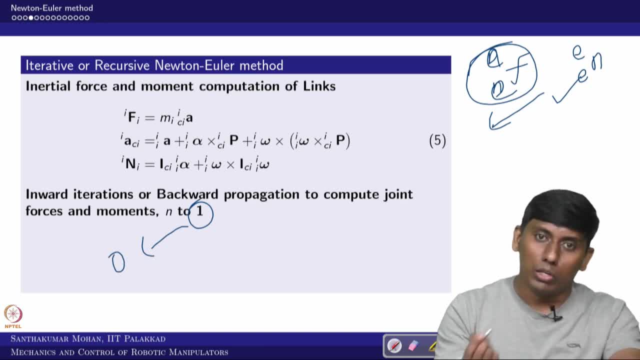 shaking forces. so whatever is transmitted to the base, whatever transmitted as a moment to the base, that would be shaking moments. So if you actually like, go to zero that. so f: 00 and n: 00, that would be shaking force and moment. right now we are bothering about only motion dynamics. 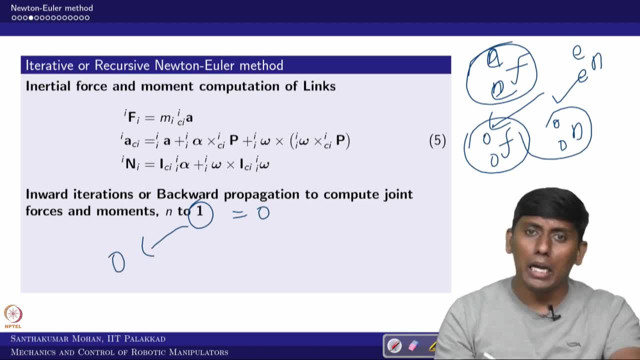 We will actually like do it. one simple advantage I want to tell here: so the comparison between Lagrangian Euler and Newton Euler. the Newton Euler would give all three. you can say axis, force component and moment component. So in that sense, when you want to do the structural dynamics or you want to do a design, so these 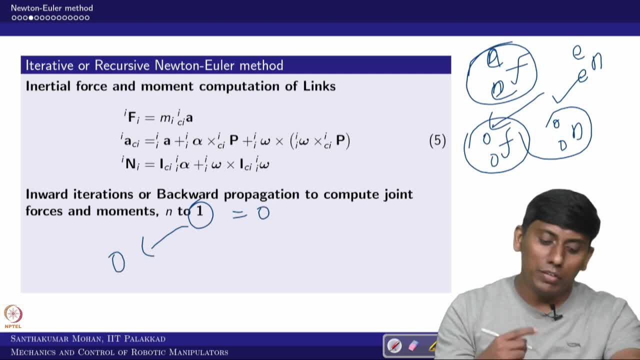 equations would be beneficial, okay, so that is why we are actually, like always, encouraged to use Newton Euler rather than the Lagrangian Euler. okay, But we will be seeing in the next lecture what is the comparison between these two. but any, now you can get this idea. 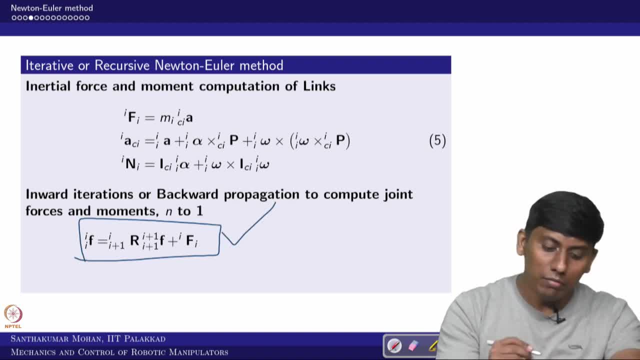 So now this is what the equation which is we have, because when you talk about this is the link, so this link would be having fi, because ith frame. this is actually like f, i plus one, i plus one, But this I have initiated force. now, when you see this point, if you assume that this is, 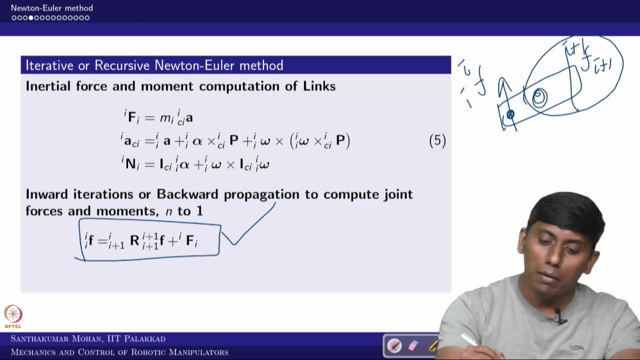 a dynamic equilibrium or equilibrium, two forces sum supposed to be equal to this right. so that is what we are writing it here. The same way, if you talk about moment, so there is a moment here, so that moment would be having a- you can say- couple happening here. that also will come. so that is what you can. 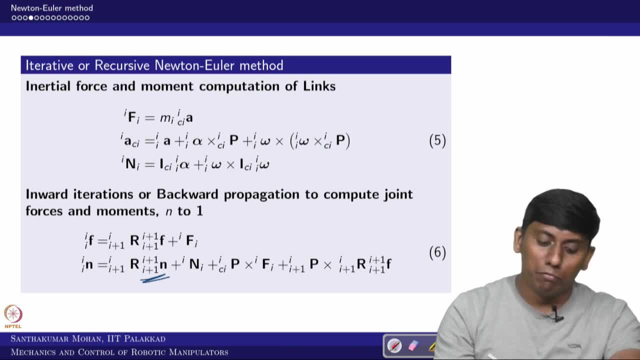 see. So this is actually like from the you can say forth going joint, or you can say the joint which is in the front, and this is actually like a centroidal force is actually like how much couple it will generate. similarly, the end of factor force, how much couple it can. 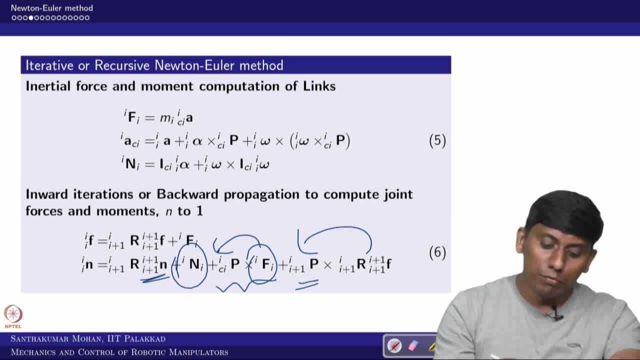 produce and this is the initial moment. okay, So now you do not have initial efforts. okay, So if you do not have initial effort, it is a static equilibrium. now, if you consider that would be the dynamic case, now, you are clear. 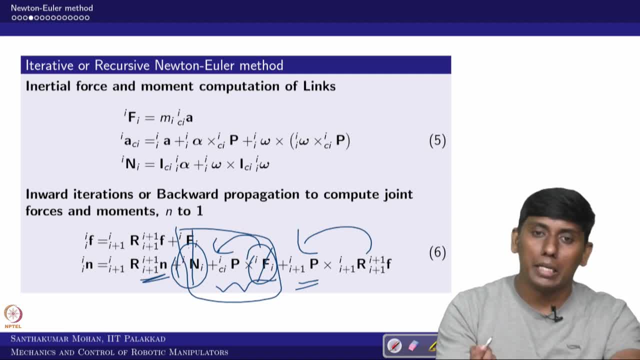 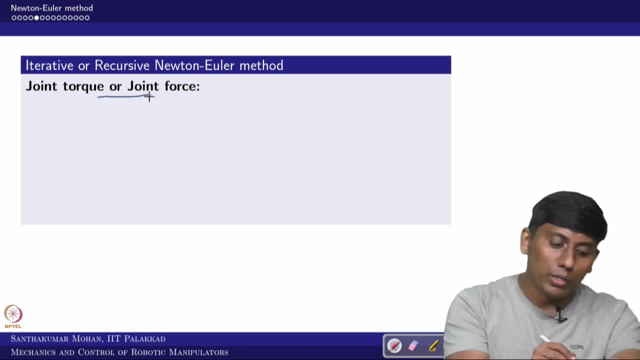 right, So the inertia forces: if you include that become dynamic case. if you ignore that would be a static case. it is very straight forward, right? So now we will actually like try to calculate the dynamic case. calculate So what would be the joint arc or joint force if it is actually like a linear? 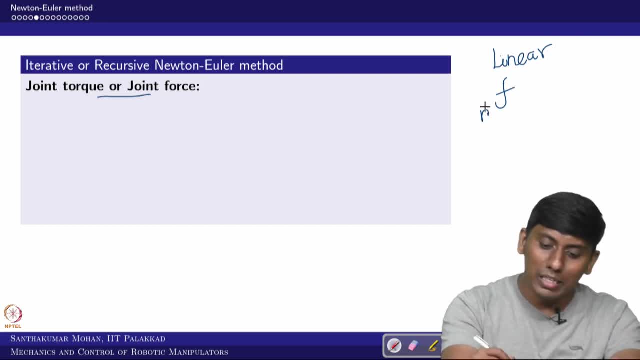 joint. So then the f corresponding to you can say that ith joint. the third quantity in the sense z axis component would be your tau i. if it is a rotary, So then the n of 3, the third component of i, would be your tau i. that is what I am writing in a. you can say: 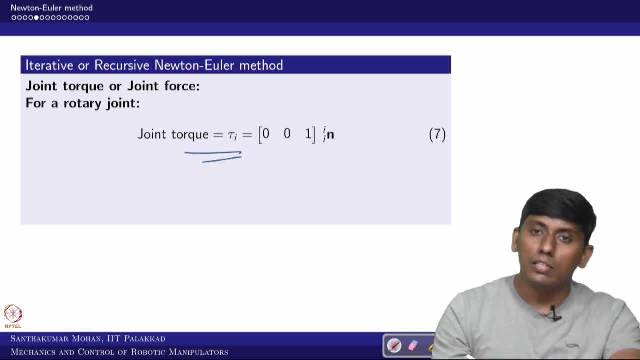 proper vector form So you can actually like see it this. So now, this is actually, like you can say, row vector and this is actually like column vector. So now, if you multiply, that would be coming the third component, which is given as a torque, which is a rotary joint. 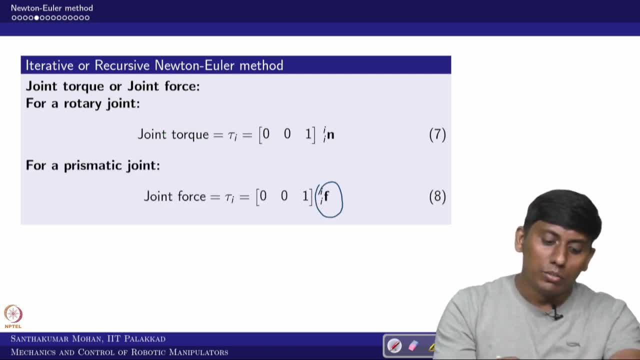 If it is a prismatic joint, so that would be the force vector, So then this would be a joint force. the third axis or the third component of, you can say force vector would be your tau. So you can actually like see one simple example, then we will actually like close this particular. 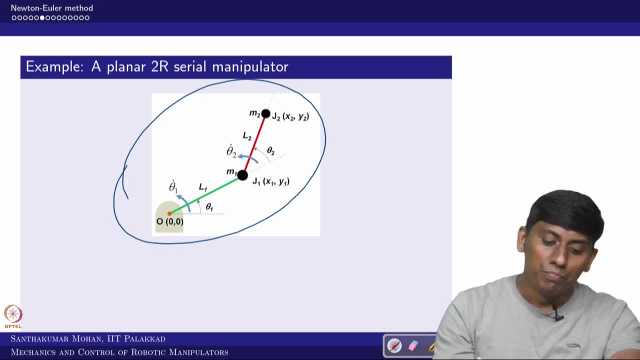 lecture. for that we have taken the same picture which we have shown in the previous lecture. as Newton, you can say Lagrangian Euler- The same thing we are using for Newton Euler also. only thing, this is actually like you have to fix the frame. So I assume that this is. 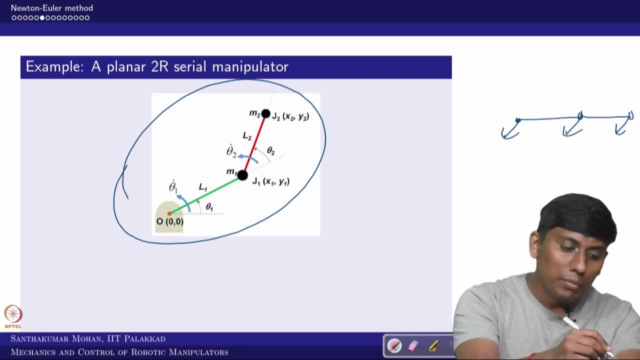 the frame arrangement, So I am actually like keeping it. this is z 0- 1.. So this is actually like a theta 1 and this is theta 2, this is z 2 and this is z 3, this is 2 and this is. 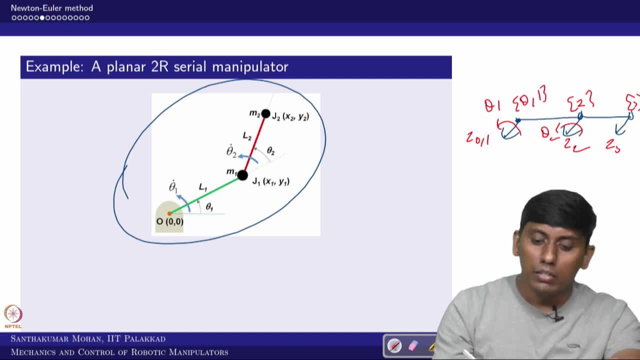 3 and this is 0 and 1.. So now, what one can actually like see where is the x axis go. this is x 1 and 0, and this is x 2 and this is x 3.. So, in the sense, what one can actually like find, you can actually like find the what you. 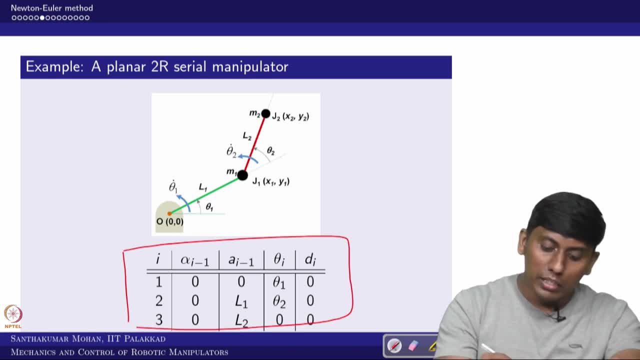 call the d h parameter. So the d h parameter. I will just to show it here for your purpose, because last time I have drawn which is actually like gone out, So this is z 0, 1 and this is z 2, this is z 3.. So I am just to showing it how this x 0, 1 goes, this is x 2 and this: 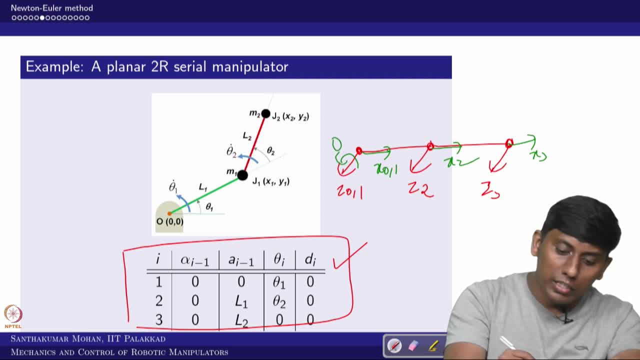 is x 3. ok, So now this is actually like theta 1 and this is theta 2. right now we assume theta 1 and theta 2 are 0, but that is active joint, So in the sense you can see a 0 and. 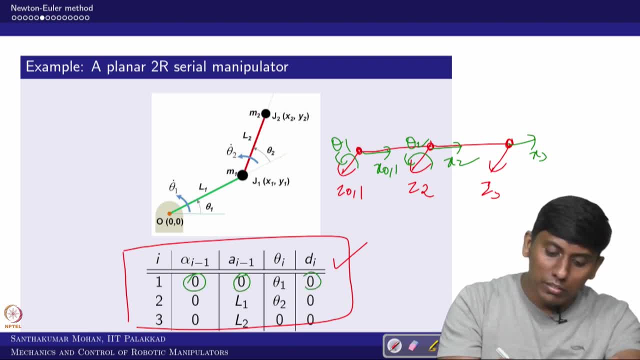 1 are same point in the sense both distance. So both distance are 0 and both are parallel. the angle is 0, but x, 0 and 1 are parallel, but there is active joint. that is why theta 1 is coming in the sense 0 plus theta 1.. 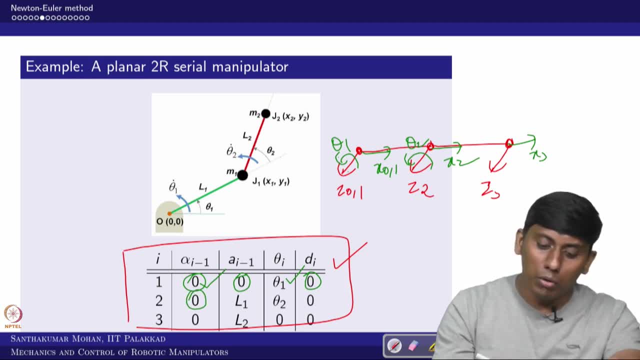 Second: similarly, there is no Angle between z 1 and z 2, but there is a distance along x 1, that is l 1 and that is the active joint theta 2, and there is no distance along z axis. So these are 0, right? So now? 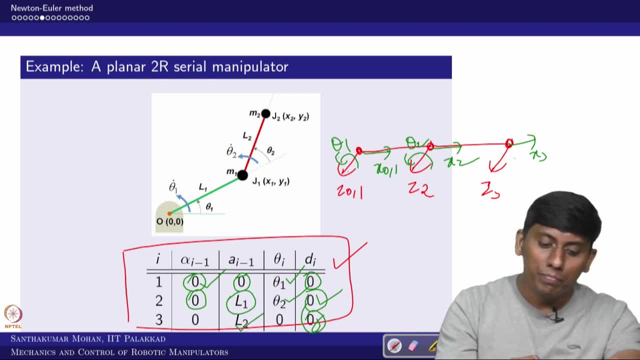 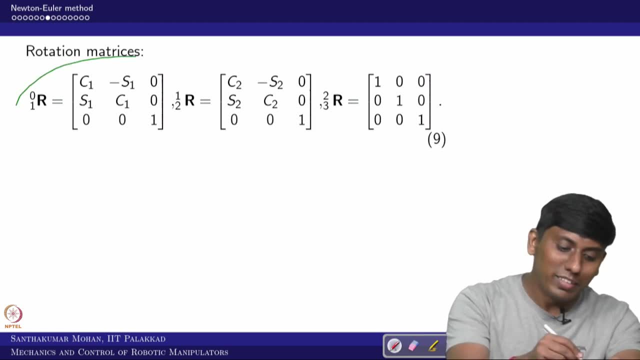 you can see, this is actually like passive joint, So only l 2 comes. So now, based on this, what one can do, we can actually like get the individual transformation matrix from there. you can extract the rotation matrices, ok, And you can. 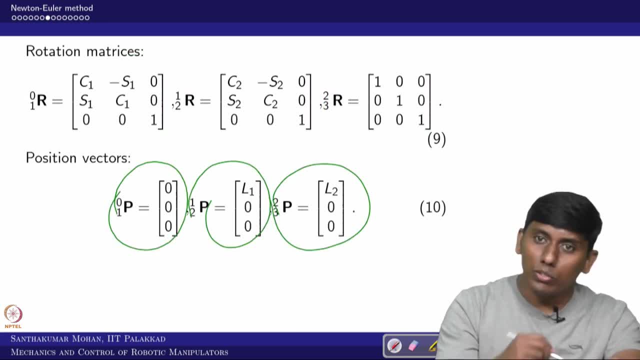 You can actually like extract position vectors. in addition to that, you need one more. what one more? So you need to actually like extract the centroidal location because you are actually like trying to find out v, c, i and a c i right. So because you need to calculate the initial. 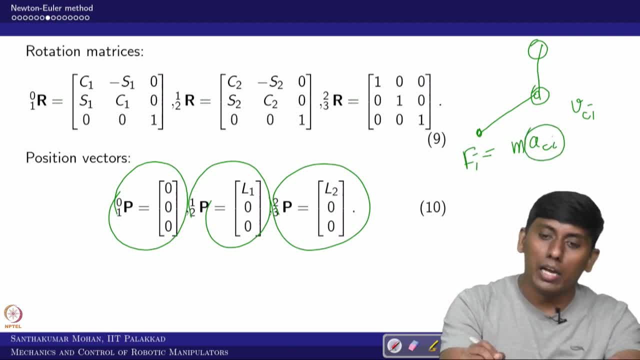 you can say forces right, f, i. So this, a c i. you need to calculate for that. you need to know the p c i. in this case, what would be the p c i? So you can see that this is actually like along x. So this is the mass concentrated, So I will show it here. So 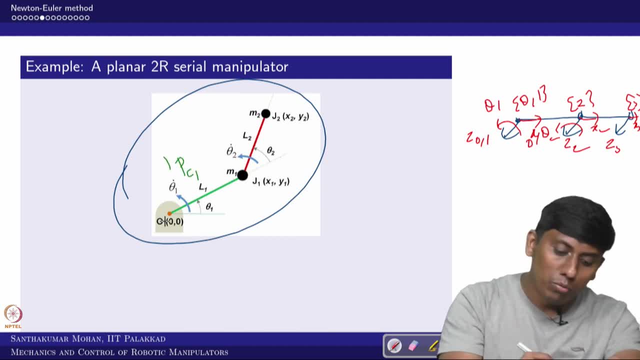 what is actually like p c 1 with respect to 1, 1 is here z 1.. So this is the first centroidal location, So that is along x 1.. So in the sense the p c 1 with respect to 1 would be: 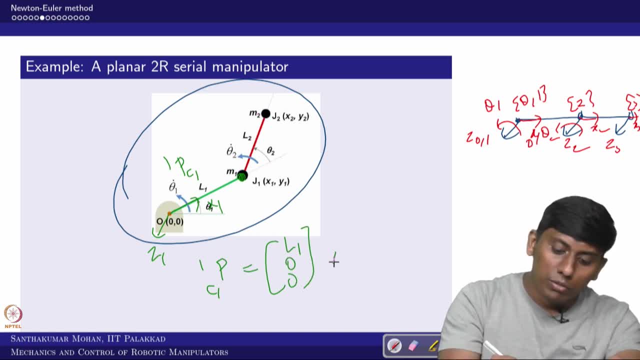 x 1, l 0,, 0 right, So p, c 2 with respect to 2, this is part two, z two. So what is So? what is this? This is actually like x 2.. So then it is actually like L 2, 0, 0.. So. 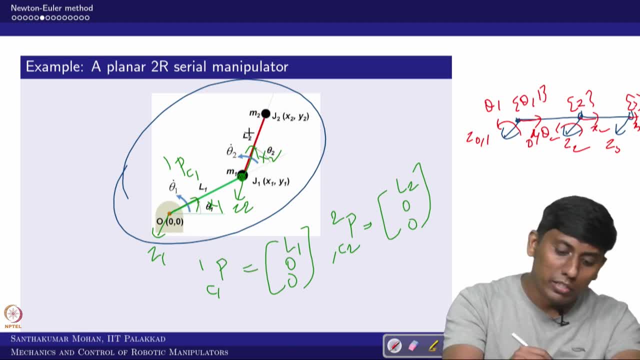 please be clear. So now, for example, the centroid is coming here, So then this is actually like L, c, 2.. So now you have a triangular link like this: This is z 2 and your centroid somewhere coming here. So then you can see like this is x axis and this is actually like 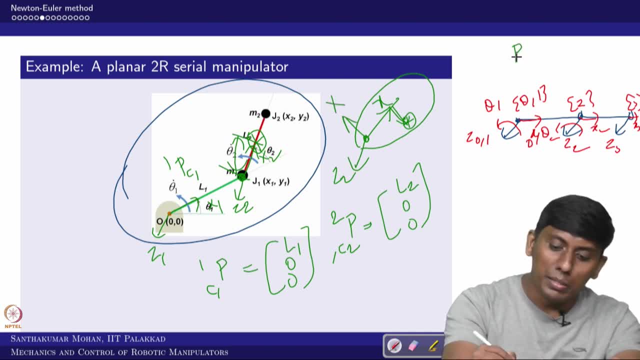 this is your y axis, So this is down. So what would be the P c in this case? So 2, 2.. So this would be x and minus y, the value I say, and 0, right, So you be clear. So. 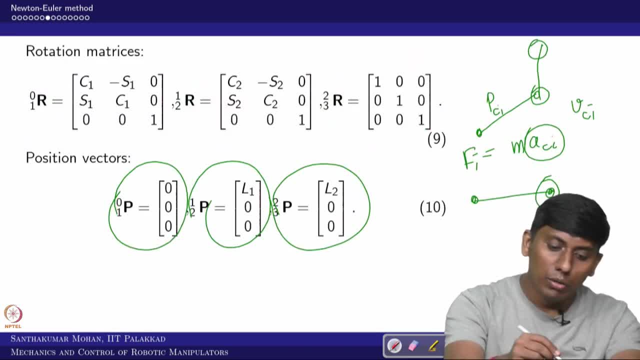 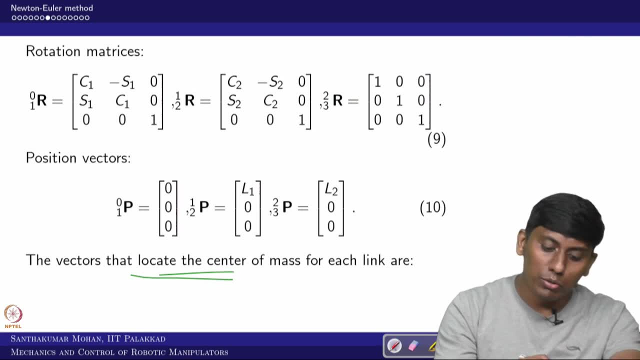 this is actually like with respect to link, So now that also we are actually trying to find out. So in this case it is actually like P c 1 would be, L 1 0, 0, P c 2 would be. 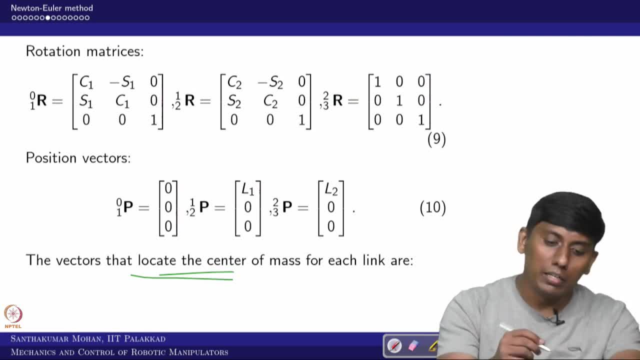 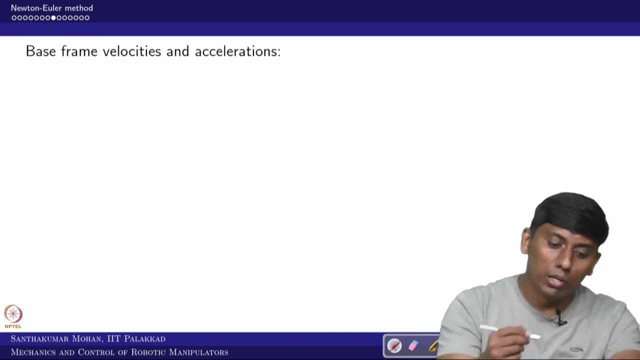 L 2 0, 0.. In this case only two link, So two link centroidal. we have actually a calculator right. Once you calculate it, then we can go forward. For the forward propagation we calculate the angular velocity linear. 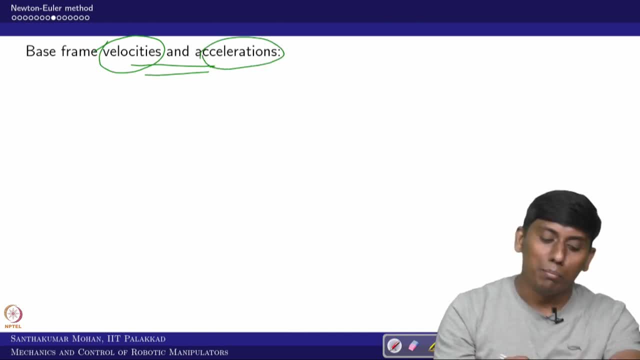 velocity and acceleration. In this case, linear velocity is not important. So we will calculate angular velocity, angular acceleration and linear acceleration Further. we will end with linear acceleration at centroidal location. So that is what we are trying to do. So